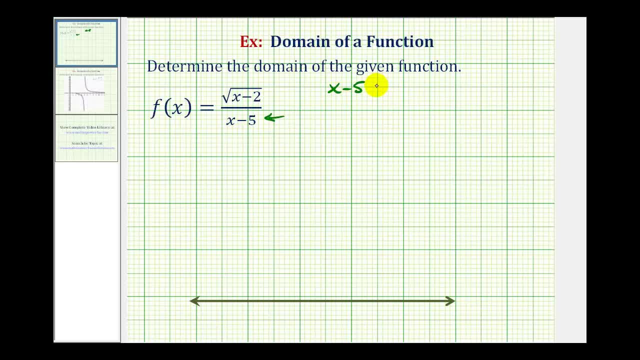 So to show this, let's set x minus five equal to zero. If we solve this, we can see: x equals five would make the denominator equal to zero and therefore we must exclude this value, because that's when we'd have division by zero. 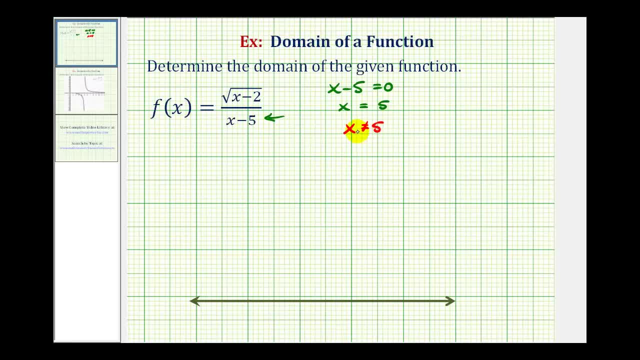 So x cannot equal five is one restriction on the domain. Now let's consider the numerator. In order for the numerator to be a real number, the number underneath the square root cannot be negative, meaning it must be greater than or equal to zero. 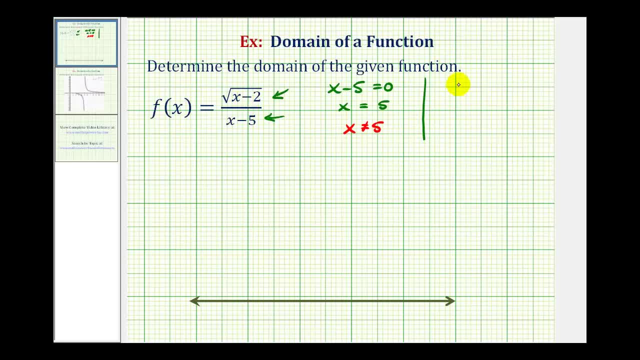 So the next restriction is: x minus two must be greater than or equal to zero again, in order for the numerator to be a real number. So if we solve this for x, we have x is greater than or equal to positive two. This is the second restriction on our domain. 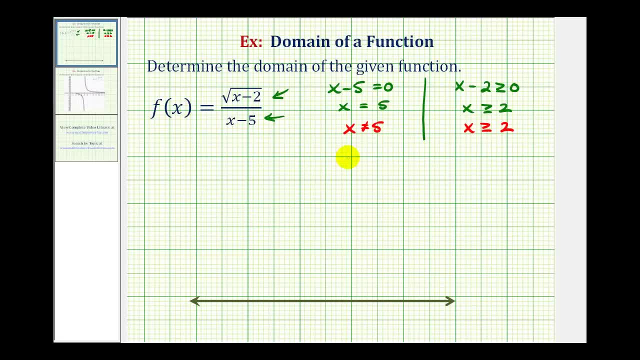 So there are several ways to express the domain. One way would be to say: the domain is when x is greater than or equal to positive two And x does not equal five. But let's also graph this domain. So we'll start by labeling our number line. 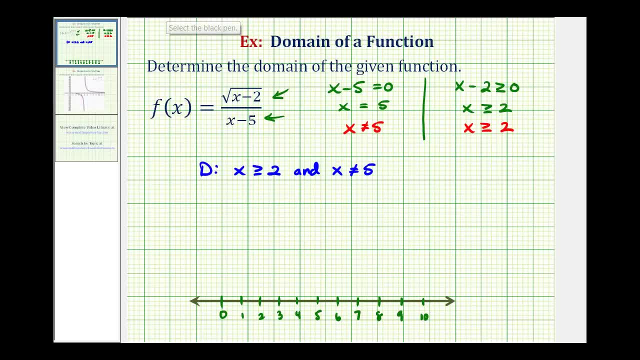 Let's start with to exclude five from the domain. we'll make an open point on the number line at positive five And then we'll graph the inequality. x is greater than or equal to positive two. keeping in mind x can't equal five. 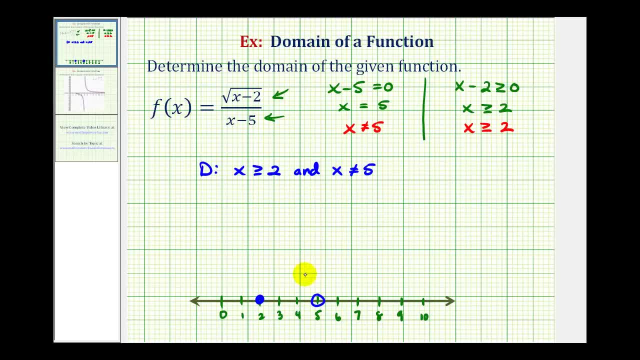 So we'd have a closed point on positive two And then an arrow to the right. But because we have to exclude five, we would draw our arrow from here to the open circle on five and then continue it to the right of positive five. 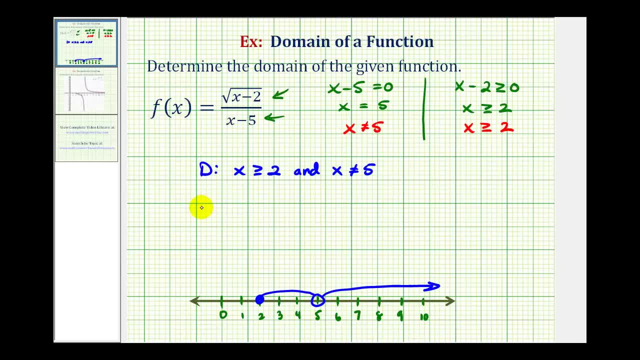 This would be the graph of the domain of the function. Let's also list the domain of the function using interval notation To help us do this. we know, as we continue right, we're going to approach positive infinity. So we have two intervals here. 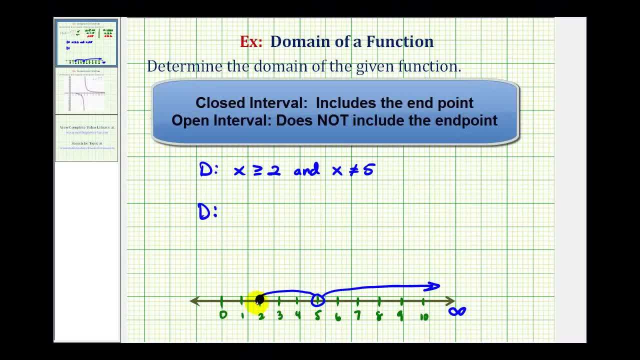 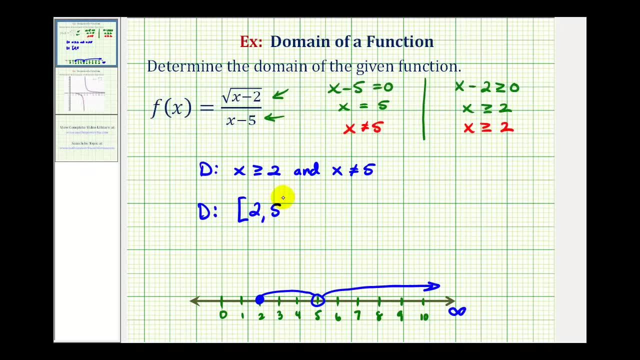 We have the interval from two to five, where the interval is closed on two and open on five. So we'd have a square bracket on two and a parenthesis on positive five union, And then we have the interval from five to infinity, open on five.